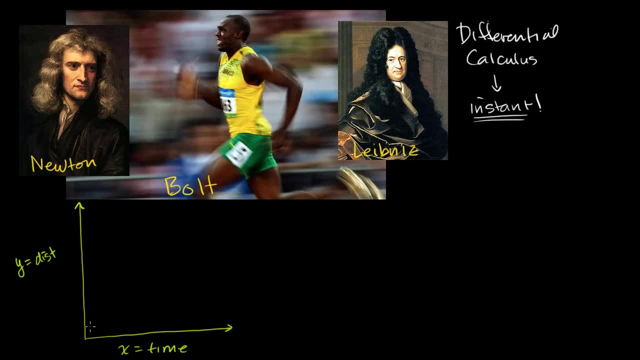 And so if we were to plot Usain Bolt's distance as a function of time, well, at time zero, he hasn't gone anywhere. He is right over there, And we know that this gentleman is capable of traveling 100 meters in 9.58 seconds. 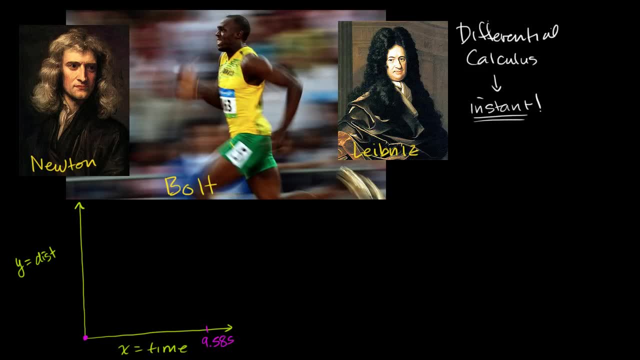 So after 9.58 seconds- we assume that this is in seconds- right over here he's capable of going 100 meters, 100 meters, And so, using this information, we can actually figure out his average speed, His average. let me write it this way: 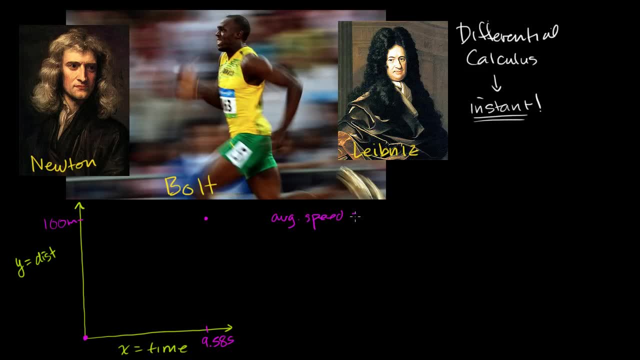 his average speed is just going to be his change in distance over his change in time. And using the variables over here we're saying y is distance. So this is the same thing as change in y over change in x from this point to that point. 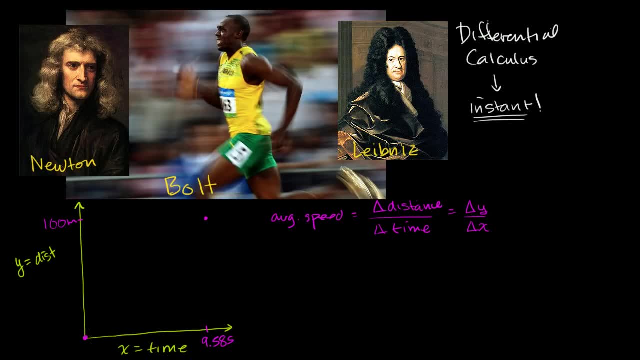 And this might look somewhat familiar to you from basic algebra- This is the slope between these two points. If I have a line that connects these two points, if I have a line that connects these two points, this is the slope of that line. 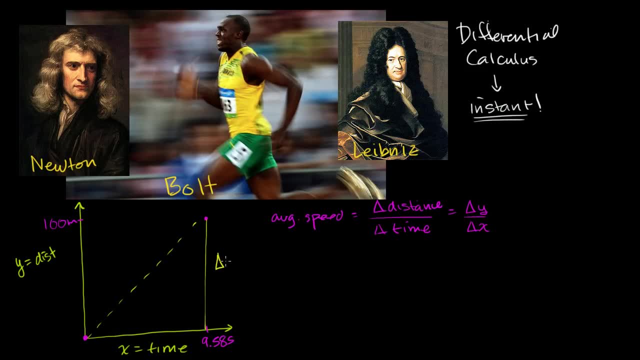 The change in distance is this: right over here. Change in y is equal to 100 meters And our change in time is this: right over here. So our change in time is equal to 9.58 seconds: 9.58 seconds. 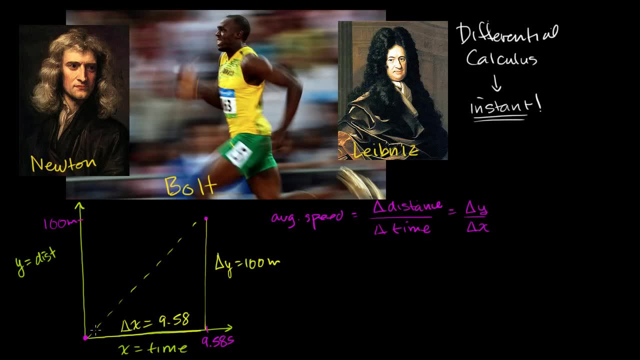 We started at 0.. We go to 9.58 seconds. Another way to think about it. the rise over the run you might have heard in your algebra class is going to be 100 meters over 9.58 seconds. 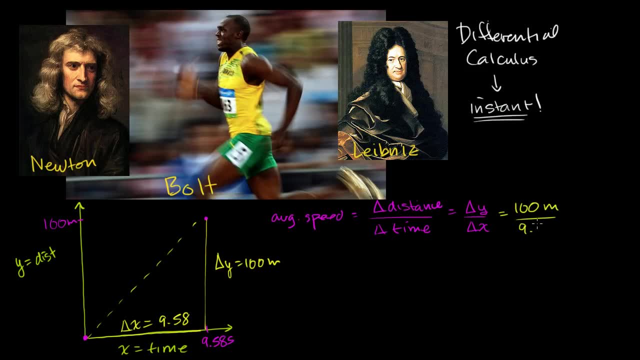 So this is 100 meters over 9.58 seconds, And the slope is essentially just the rate of change, or you could view it as the average rate of change between these two points And you'll see if you even just follow the units. 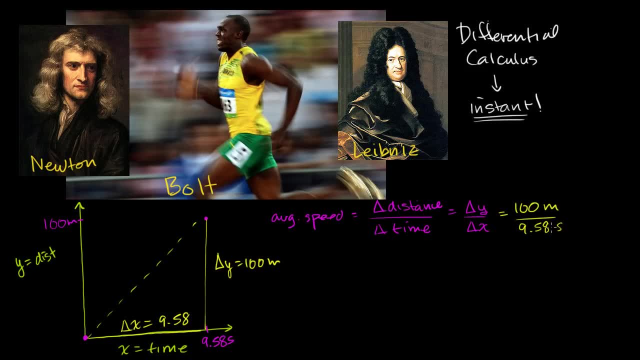 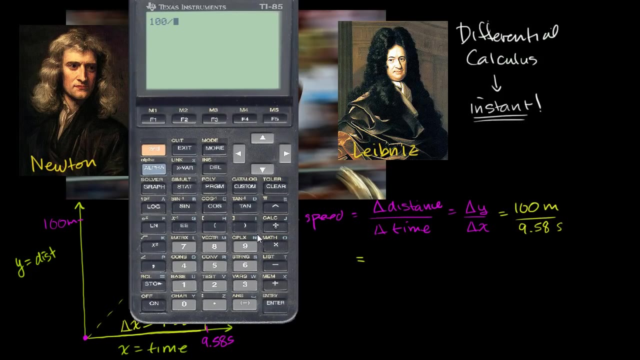 it gives you units of speed. here It would be velocity. if we also specify the direction And we can figure out what that is. Let me get a calculator out. I'll get the calculator on the screen. So we're going 100 meters in 9.58 seconds. 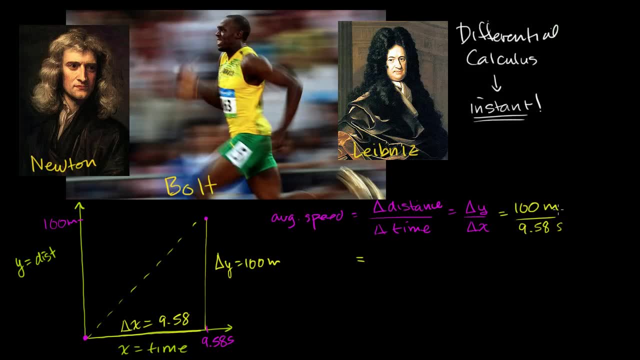 So it's 10.4.. I'll just write 10.4.. I'll round to 10.4.. So it's approximately 10.4.. And then the units are meters per second, And that is his average speed. 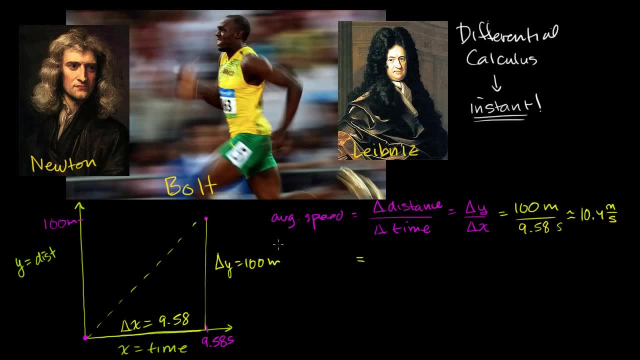 And what we're going to see in a second is how average speed is different than instantaneous speed, how it's different than the speed he might be going at any given moment. And just to have a concept of how fast this is, let me get the calculator back. 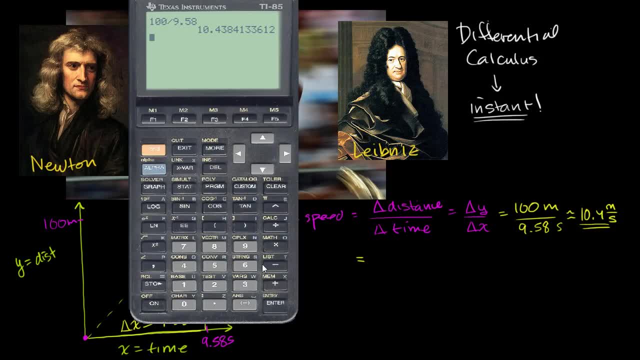 This is in meters per second. If you want to know how many meters he's going in an hour, well, there's 3,600 seconds in an hour, So he'll be able to go this many meters 3,600 times. 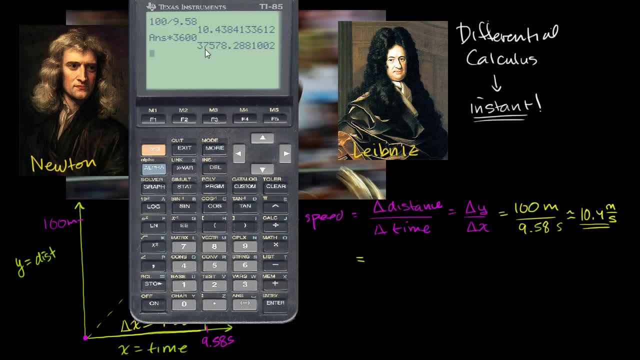 So that's how many meters he can. if you were able to somehow keep up that speed in an hour, this is how fast he's going, meters per hour. And then if you were to say how many miles per hour, there's roughly 1,600. 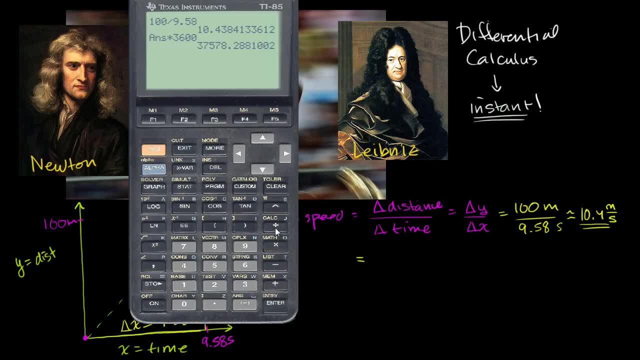 And I don't know the exact number, but roughly 1,600 meters per mile. So let's divide it by 1,600.. And so you see that this is roughly a little over 23,. about 23 and 1 half miles per hour. 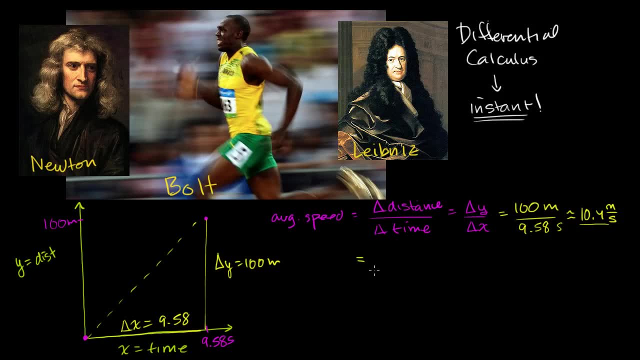 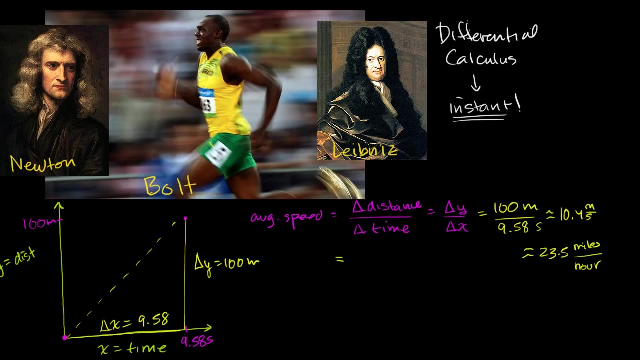 So this is approximately. I'll write it this way: this is approximately 23.5 miles per hour. OK, Let me scroll over so I don't have to bunch that. Miles per hour, And relative to a car, not so fast. 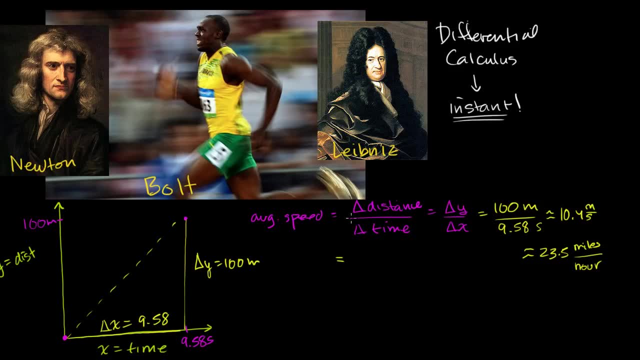 But, relative to me, extremely fast. Now to see how this is different than instantaneous velocity, let's think about a potential plot of his distance relative to time. He's not going to just go this speed immediately. He's not just going to go as soon as the gun fires. 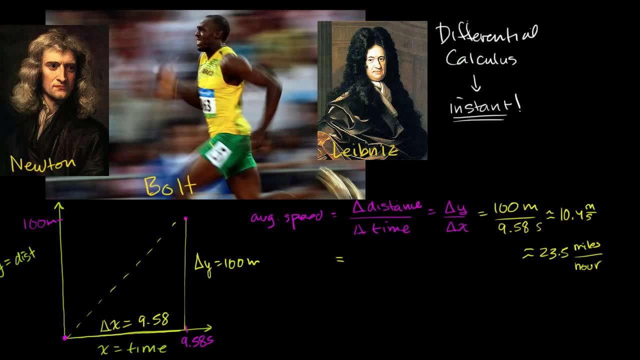 He's not just going to go 23 and 1 half miles per hour. all the way He's going to have to accelerate. So at first he's going to start off going a little bit slower, So his slope is going to be a little bit lower. 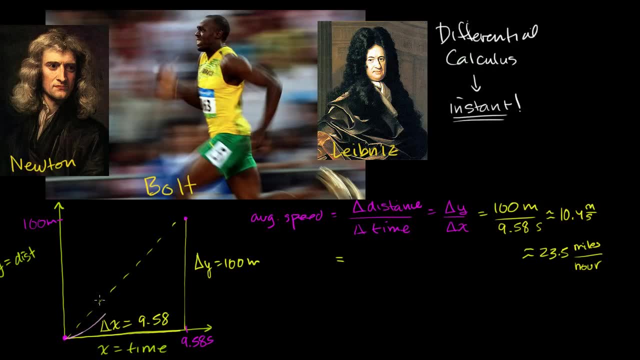 than the average slope. He's going to go a little bit slower, Then he's going to start accelerating And so his speed- and you'll see the slope here is getting steeper and steeper and steeper And then maybe near the end he starts tiring off a little bit. 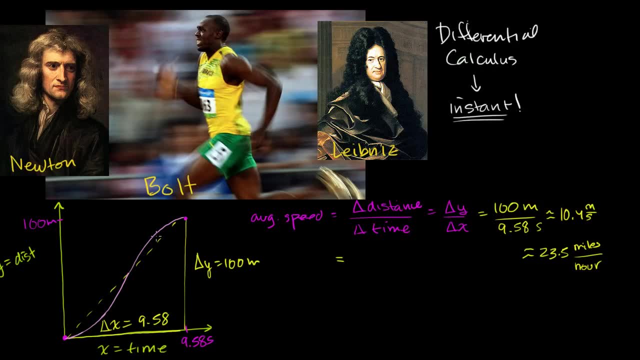 And so his distance plotted against time might be a curve. that looks something like this, And what we calculated here is just the average slope across this change in time, But we could see it at any given moment. the slope is actually different In the beginning. 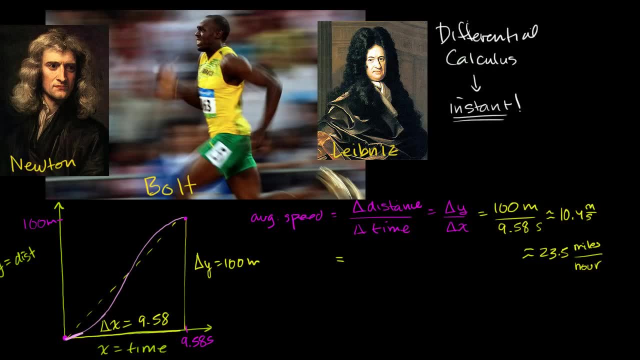 He has a slower rate of change of distance Then over here. then he accelerates over here. It seems like his rate of change of distance which would be roughly, or you could view it as the slope of the tangent line at that point. 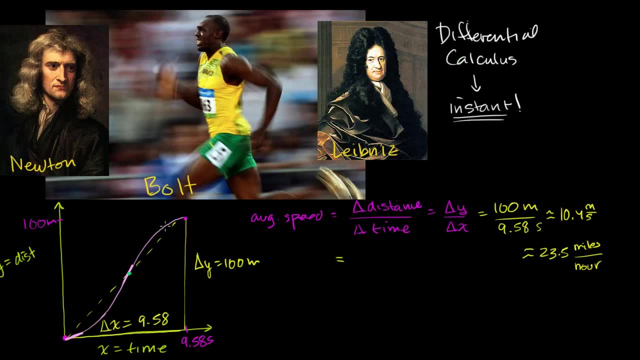 it looks higher than his average And then he starts to slow down again And when you all average it out, it gets to 23 and 1 half miles per hour. And I looked it up: Usain Bolt's instantaneous velocity- his peak instantaneous velocity- is actually: 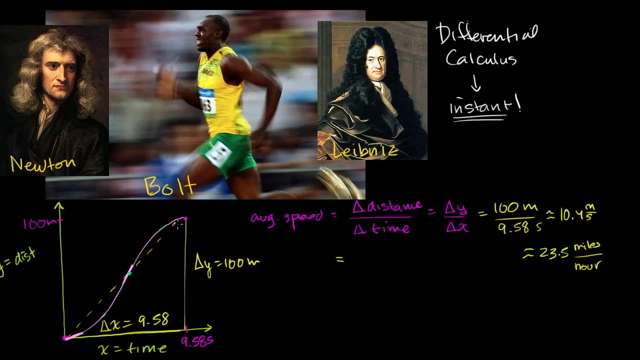 closer to 30 miles per hour. So the slope over here might be 23 whatever miles per hour, But the instantaneous, his fastest point in this 9.58 seconds, is closer to 30 miles per hour. But you see, it's not a trivial thing to do. 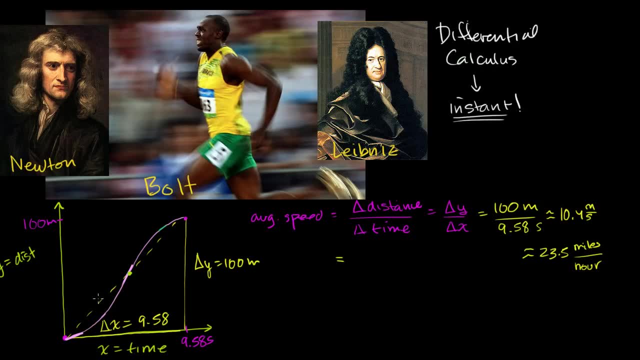 You could say, OK, let me try to approximate the slope right over here. And you could do that by saying, OK, well, what is the change in y over the change of x right around this? So you could say, well, let me take some change of x. 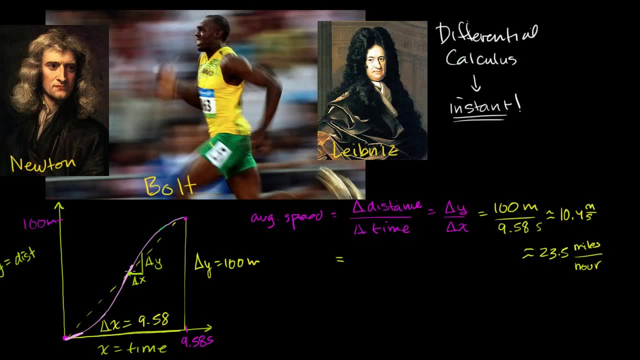 and figure out what the change of y is around it or as we go past that. So you get that, But that would just be an approximation, because you see that the slope of this curve is constantly changing. So what you want to do is see what. 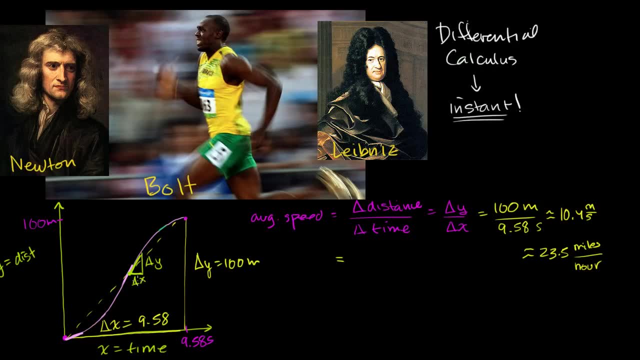 happens as your change of x gets smaller and smaller and smaller. As your change of x gets smaller and smaller and smaller, you're going to get a better and better approximation. Your change of y is going to get smaller and smaller and smaller. So what you want to do, and we're 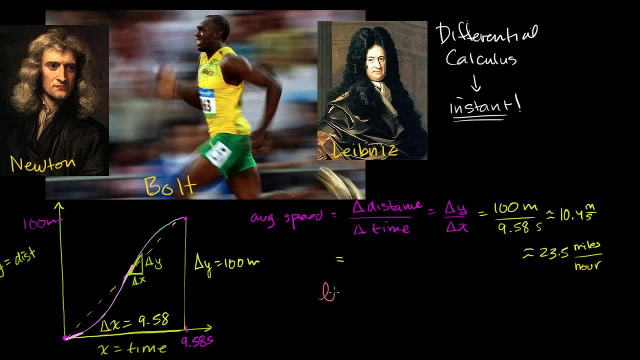 going to go into depth into all of this and study it more rigorously. is you want to take the limit, as delta x approaches 0, of your change in y right Over your change in x, And when you do that, you're going? 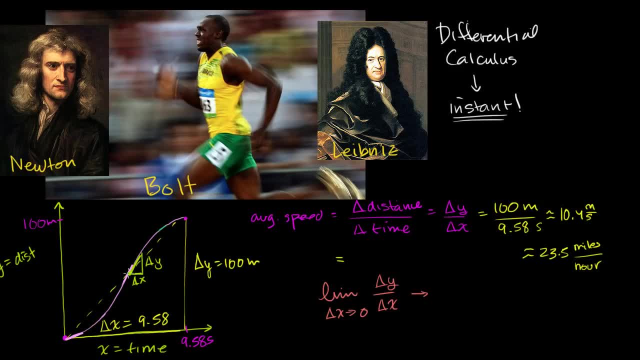 to approach that instantaneous rate of change. You could view it as the instantaneous slope at that point in the curve, or the slope of the tangent line at that point in the curve, Or, if we use calculus terminology, we would view that as the derivative.